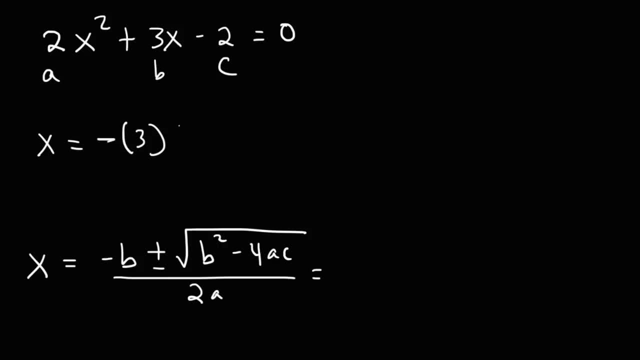 x is equal to negative b, b is positive 3, plus or minus the square root of b squared. so that's 3 squared minus 4 times a. a is 2, times c, which is negative 2, all divided by 2a or 2 times 2.. So we have negative 3 plus or minus the square root. 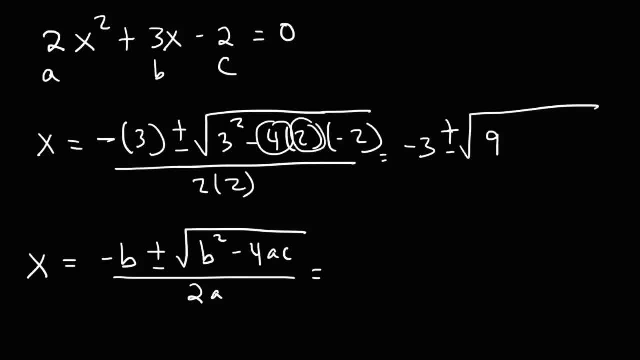 3 squared is 9, negative 4 times 2 is negative 8, and negative 8 times 2 is negative. 8, times negative 2 is positive 16.. On the bottom we have 2 times 2,, which is 4.. 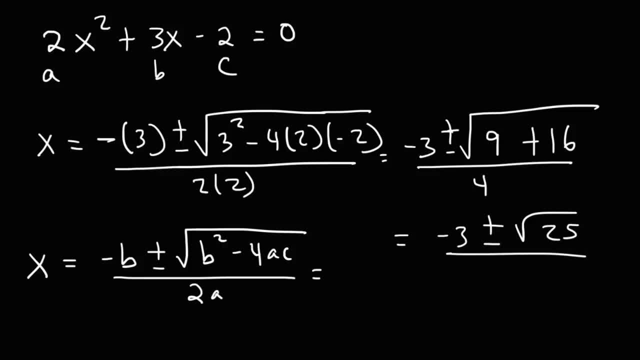 Now 9 plus 16 is 25, and the square root of 25 is 5.. So right now, that's what we have. Notice the plus or minus symbol. So we need to break this up into two parts. So we're going to have negative 3 plus 5 divided by 4,. 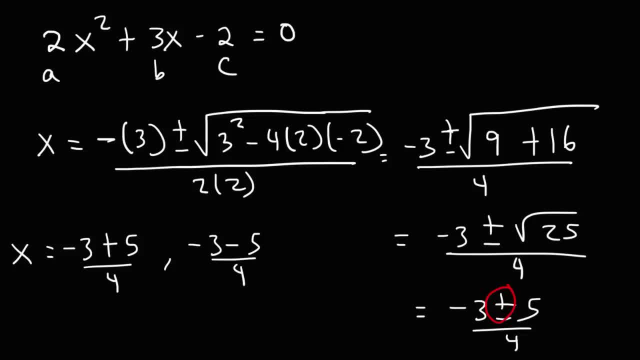 and negative 3 minus 5 divided by 4.. So we're going to have negative 3 plus 5 divided by 4, minus 5 divided by 4.. Negative 3 plus 5 is positive 2.. Negative 3 minus 5 is negative, 8.. 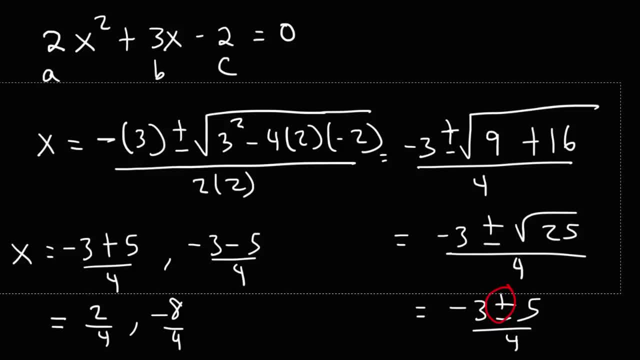 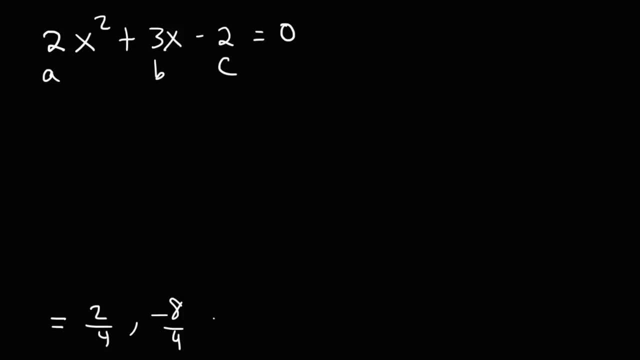 So right now we have two different answers. Now we can reduce 2 over 4 to 1 over 2, if you divide both numbers by 2.. And 8 divided by 4 is negative 2. So x can equal 1 half, or x can equal negative 2.. And so that's how you can solve a quadratic equation. 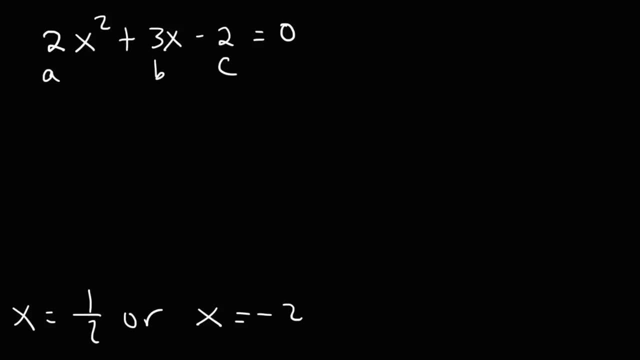 using the quadratic formula. Now if you want to check your answer, you can plug it in. Let's plug in negative 2 into this equation. So we have 2 times negative 2 squared plus 3 times minus 2, minus 2.. Let's see if that equals 0.. Negative 2 squared is negative 2 times. 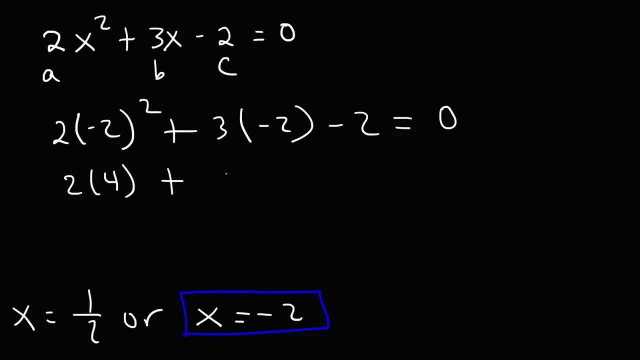 negative 2, which is 4.. 3 times negative 2 is negative 6.. Now, 2 times 4 is 8.. Negative 6 minus 2 is negative 8.. 8 minus 8 is 0. So we know that this answer works And you could try. 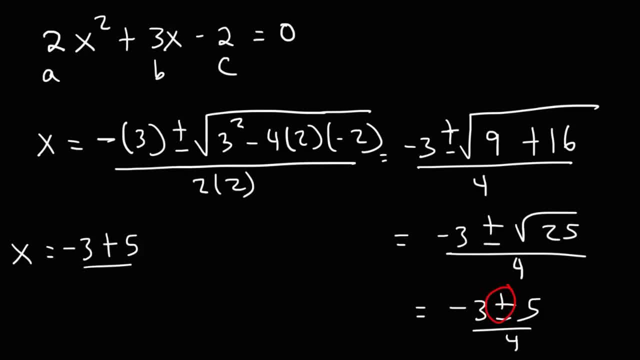 So we're going to have negative 3 plus 5 divided by 4, and negative 3 minus 5 divided by 4. So we're going to have negative 3 plus 5 divided by 4, minus 5 divided by 4. Negative 3 plus 5 is positive 2. Negative 3 minus 5 is negative 8. 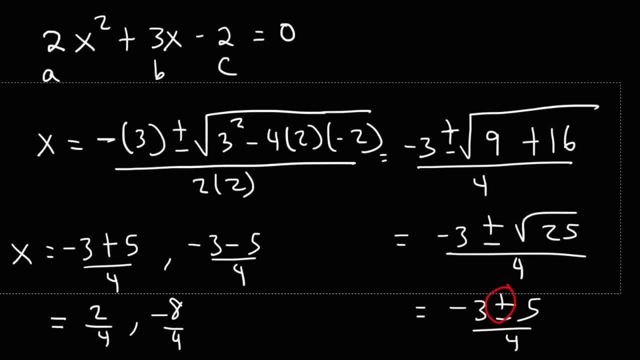 So right now, we have two different answers. 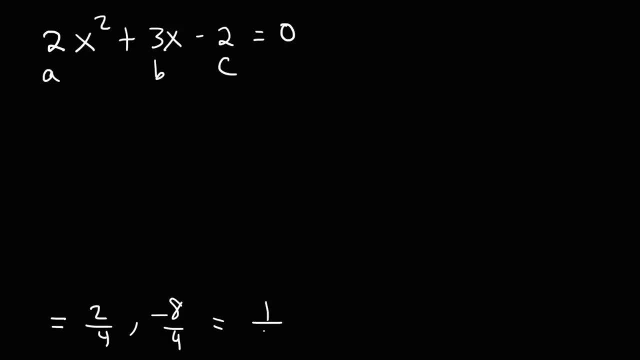 Now, we can reduce 2 over 4 to 1 over 2, if you divide both numbers by 2. And 8 divided by 4 is negative 2. 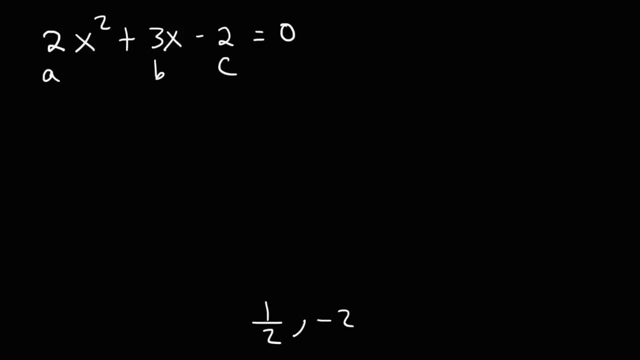 So x can equal 1 half, or x can equal negative 2. And so that's how you can solve a quadratic equation using the quadratic formula. Now, if you want to check your answer, you can plug it in. 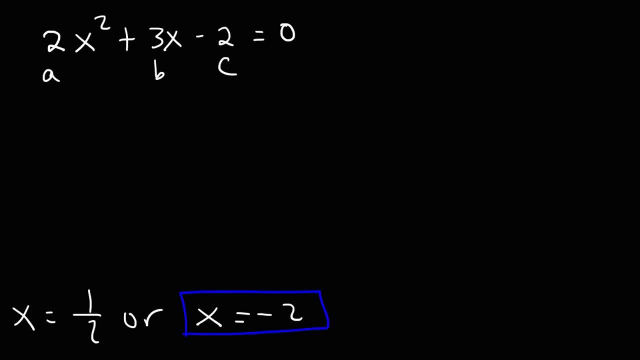 Let's plug in negative 2 into this equation. So we have 2 times negative 2 squared, plus 3 times minus 2, minus 2. Let's see if that equals 0. Negative 2 squared is negative 2 times negative 2, which is 4. 3 times negative 2 is negative 6. Now, 2 times 4 is 8. Negative 6 minus 2 is negative 8. 8 minus 8 is 0. So we know that this answer works. And you can try the 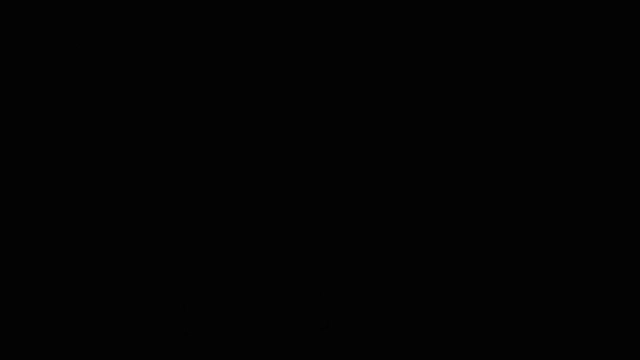 other one too. That's going to work as well. But now, let's move on to our next example. 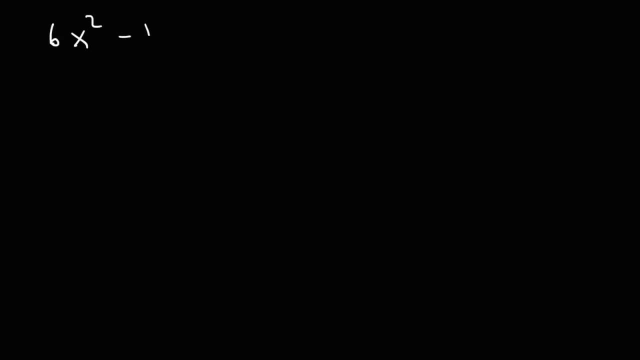 Let's say we have this particular quadratic equation. Go ahead and use the quadratic formula to get the answer. So we can see that a is 6, b is negative 17, and c is 12. So let's begin by writing the formula. So it's x is equal to negative b plus or minus the square root of b squared minus 4ac divided by 2a. 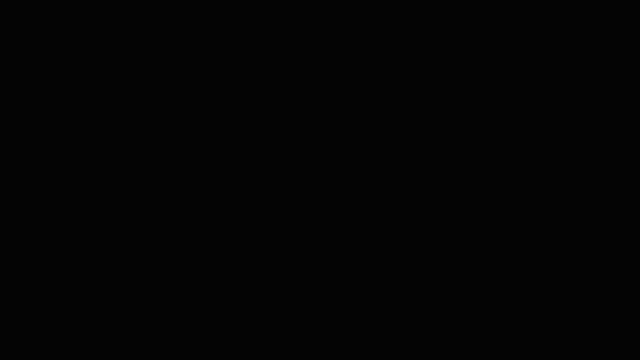 the other one too. That's going to work as well. But now let's move on to our next example. Let's say we have this particular quadratic equation. Go ahead and use the quadratic formula to get the answer. So we can see that a is 6,, b is negative 17, and c is 12.. So let's begin by. 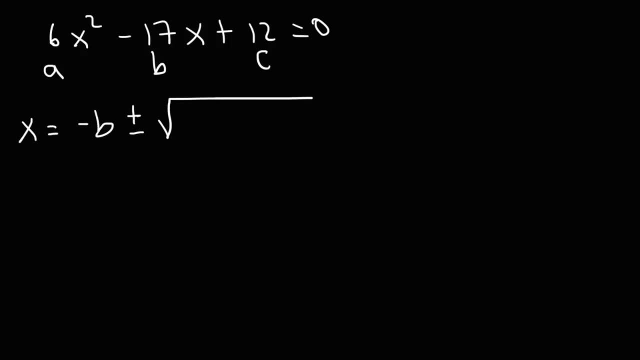 writing the formula. So it's: x is equal to negative b plus or minus the square root of b squared minus 4ac divided by 2a, So b is negative 17.. And then we have b squared. That's negative 17 squared minus 4.. A is 6.. C is: 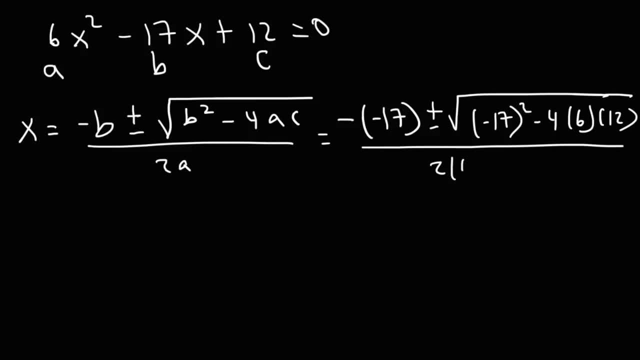 12 divided by 2a, or 2 times 6.. So we have negative times, negative 17.. That becomes positive 17.. Negative 17 squared is going to be positive 289.. And then we have negative 4 times 6, which is negative 24, times 12.. That's going to be. 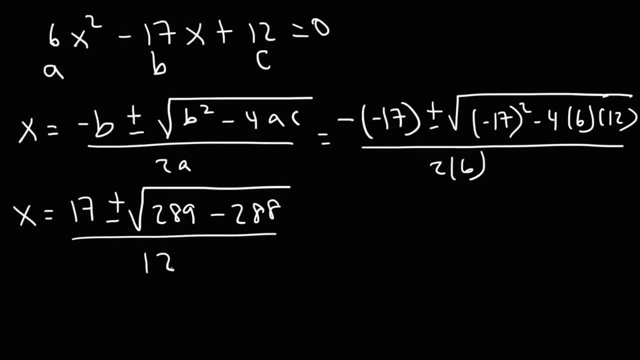 negative 288.. 2 times 6 is 12.. And inside the square root symbol we have 289 minus 288, which is the square root of 1.. And the square root of 1 is 1.. So this is what we now have. 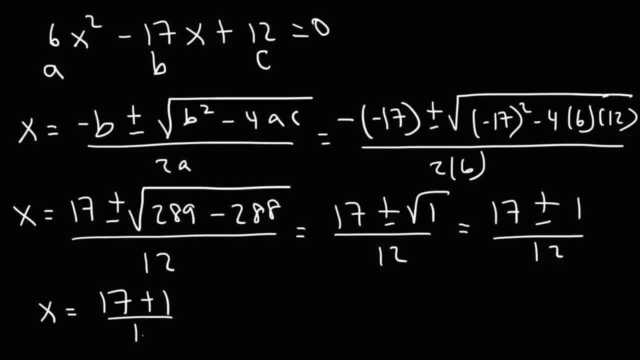 So we have 17 plus 1 over 12.. At this point, when you have the plus and minus symbol, you can break it up into two answers, And the other answer is going to be 17 minus 1 over 12.. 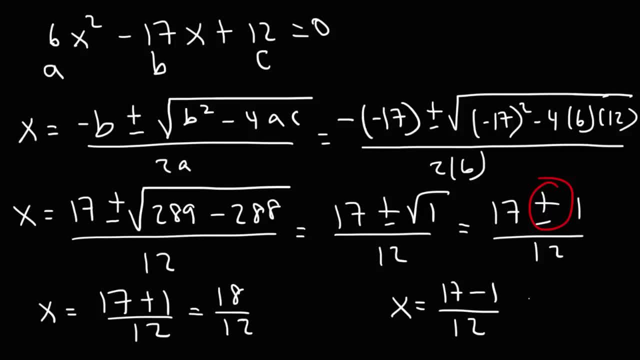 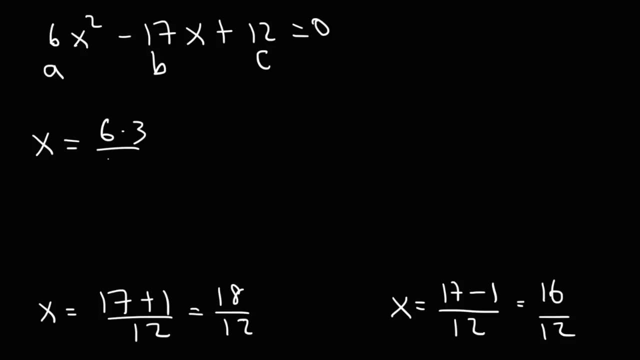 17 plus 1 is 18.. And 17 minus 1 is 16.. So now we just need to reduce those fractions. So 18 is 6 times 3.. 12 is 6 times 2.. So we have 18 plus 1 over 12.. And the other answer is going to be 17 minus 1 over 12.. 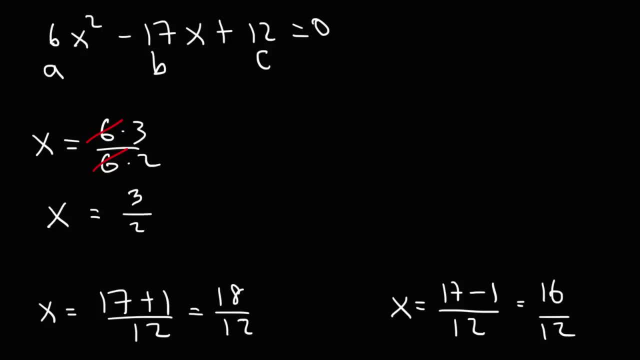 At the end of 16, we get one of our solutions as 3 over 2.. For the other one, 16,, we can write that as 4 times 4.. 12 is 4 times 3.. So canceling the 4,. 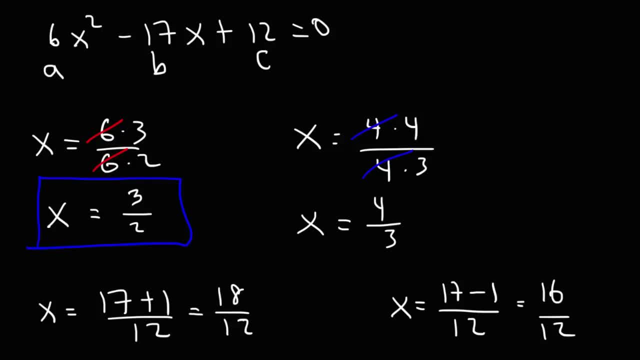 we get the other answer, which is 4 over 3.. And so that's it for this video. Now you know how to use the quadratic formula to solve a quadratic equation. Thanks again for watching. 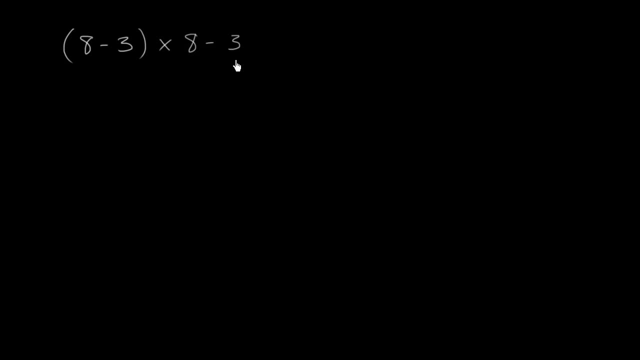 What I want to do is think about whether this expression right over here would evaluate the same way whether or not we had parentheses. So to think about that, let's first think about how it would evaluate if we have the parentheses. So, if we have the parentheses, 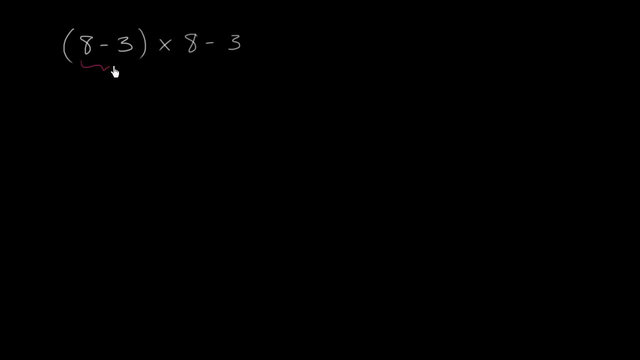 we want to do what's ever in the parentheses first, And so here we have 8 minus 3, which is equal to 5.. So this simplifies to 5 times 8 minus 3.. And now we want to do the multiplication. 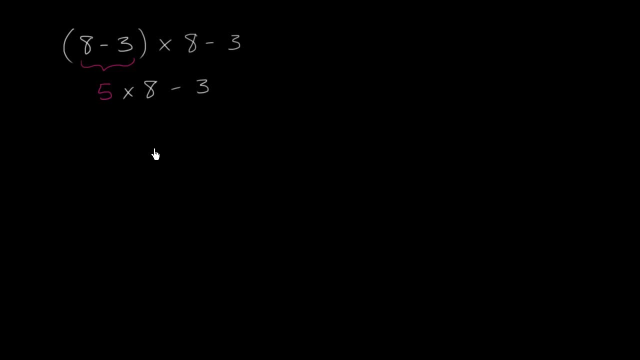 before we do subtraction. This goes back to order of operations. You do your multiplication and division first. Well, you do your parentheses first. Then, if you have multiplication, division, addition and subtraction all in a row, you want to do your multiplication and your division. 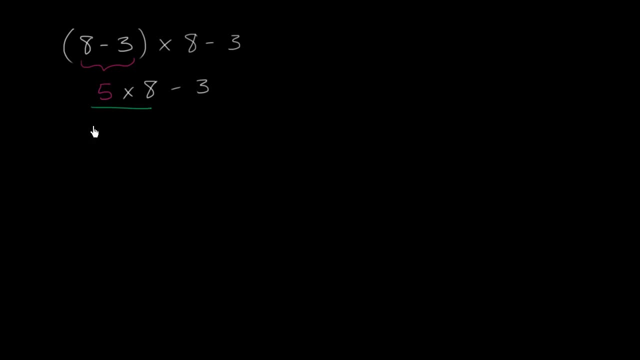 first. So here we're going to multiply 5 times 8 to get 40. And then we're going to subtract 3 to get 37. Now let's think about what this would evaluate to if we did not have the parentheses. 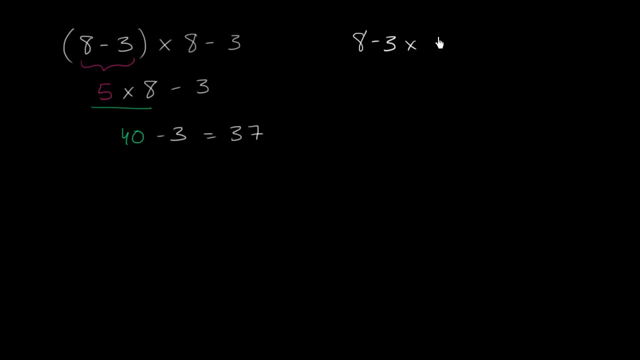 So it would be 8 minus 3 times 8 minus 3.. So we just have to remind ourselves about the order of operations. The convention is to do your multiplication first, So you're actually going to multiply the 3 times the 8 before you subtract it from this 8, and then